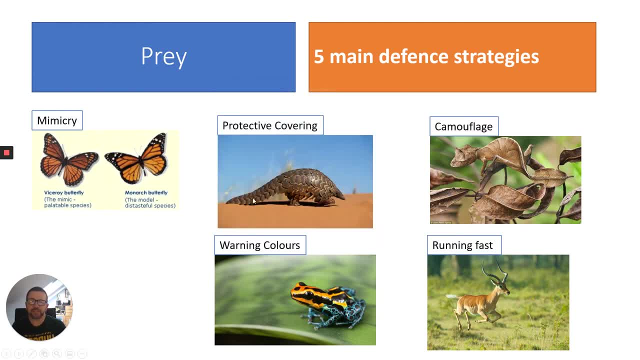 some information for you to work out what is going on. So let's look at prey defence strategies. The first thing to say is: AQA in the exam. they won't expect you to know any specific examples, So they more than likely would give you an example you've never seen before. 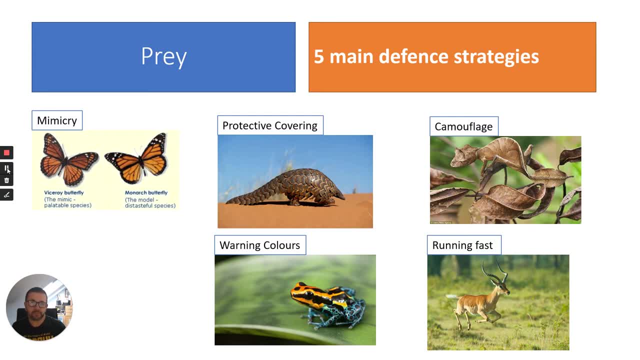 and apply your knowledge from that. So here's five main defence strategies. There are probably more, but these are quite common ones. So the first one is mimicry. So here we have a viceroy butterfly and it's a mimic and it's palatable to certain bird species, whereas a monarch butterfly is. 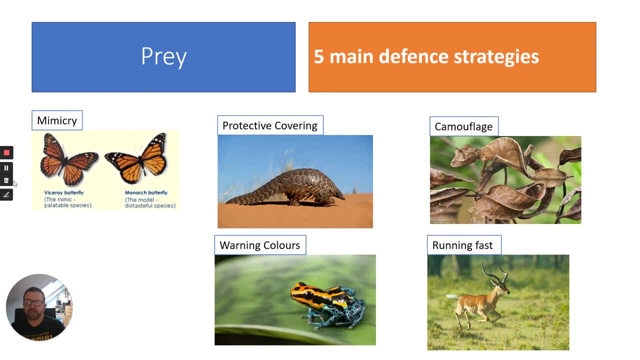 distasteful to certain species. So therefore the viceroy is benefiting from that colouration. Next one is protective covering. So there's many species that protect themselves. They can't actually outrun or shelter away from certain predators. Therefore they have protective covering. So when they are attacked it's very hard for the predator. 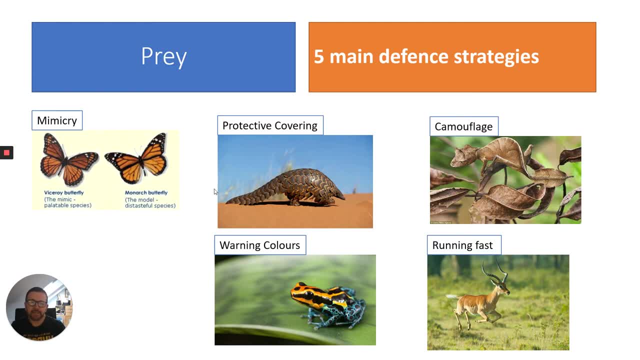 to kill them. So in this case this is a pangolin, and also another good example is in the UK is a hedgehog. Next one, camouflage, So that speaks for itself. So this reptile is extremely camouflaged and therefore will evade capture by the predator. 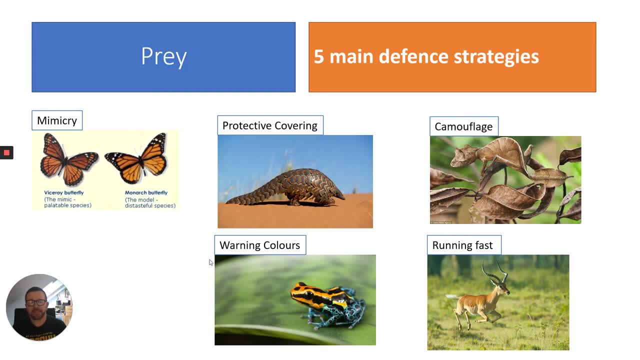 Warning colours. There's two types: Either the species is poisonous or it isn't poisonous. In this case, this is a poison dart frog and it's definitely poisonous and it's a warning colouration to generalise predators that it's not a good idea to eat this particular frog. 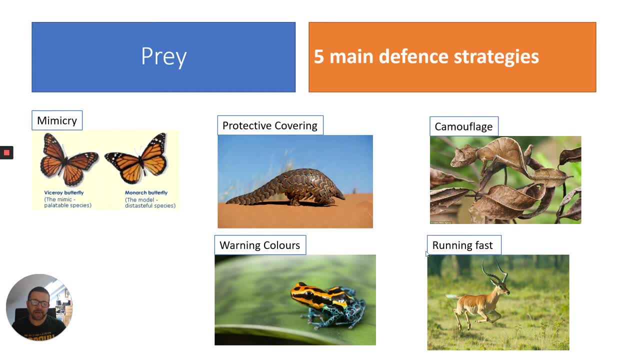 And then, finally, is running fast, So ability to outrun their predators. So this is an impala. Impalas can run extremely fast, but, more importantly, they can run fast for a sustained period of time. They're also very agile, so they can dodge out of the way. You can see, this impala has large horns as well, which 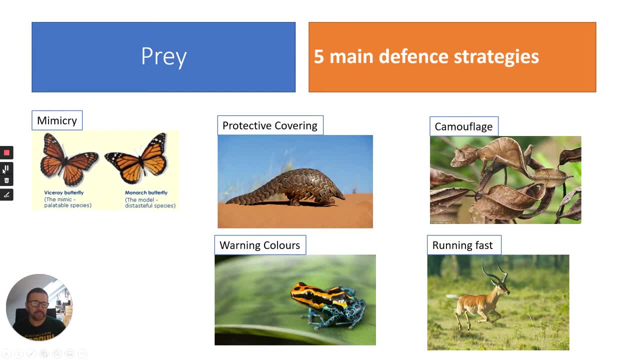 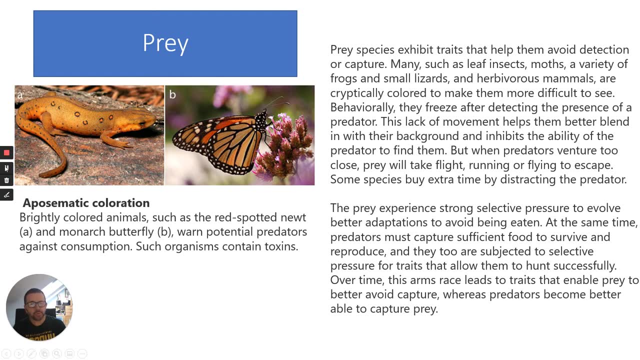 will help protect itself from being predated upon. So here's another example. So this is an example of what we call aposematic colouration. You wouldn't need to know that in an exam, but you do need to know in terms of the fact that it's an advantage, a selective advantage, to the species. 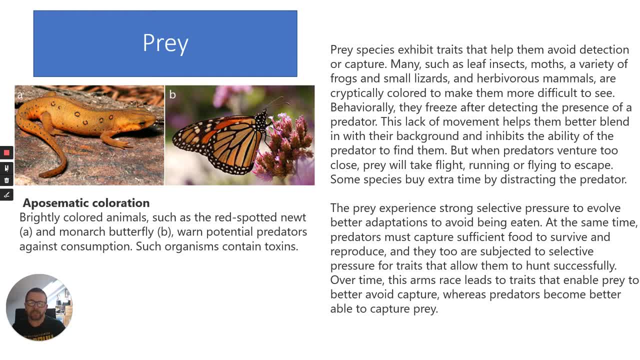 So red-spotted newton and monarch butterfly, They warn potential predators against consumption, such as organisms contain toxins, and it's very much related to something I'm going to talk about in a minute about selective pressure. So there's a move to evolve. So there's a move to evolve for better adaptations to avoid being eaten and, conversely, predators at the same time need to capture sufficient food. 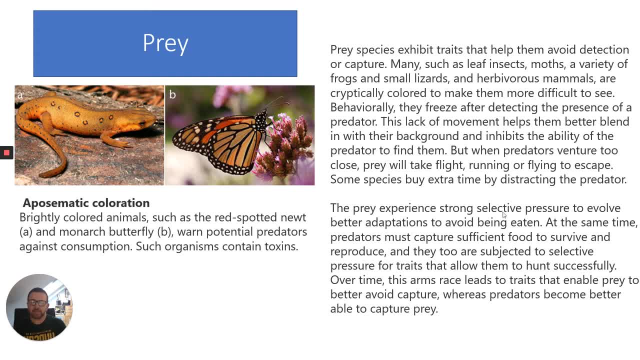 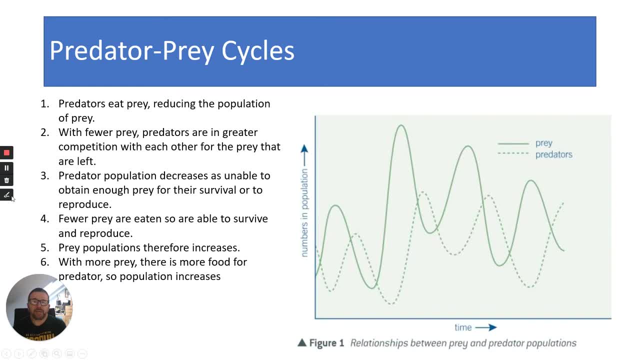 So if they have any adaptations over time, then they will have an advantage over the prey. Predator-prey cycles or predator-prey relationships usually take the same kind of shape in a graph. They usually look something like this: They will often be in an area where they are native to a species with an advantage over prey. 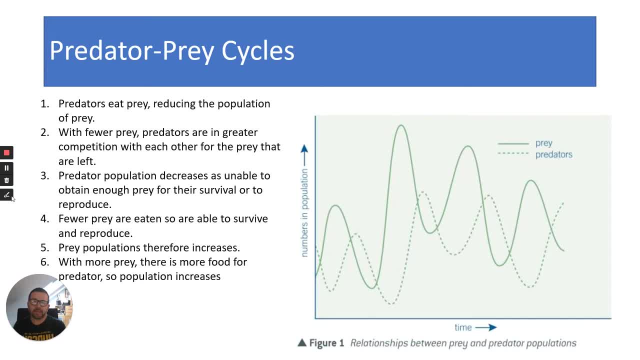 They will often be in an area where they are native to a species with an advantage over prey. obviously vary from species to species, but it's generally the same pattern, so if we just follow through, okay, so first of all, predators. so here is: the dotted line is predators and the solid green line is prey, so you can see when. 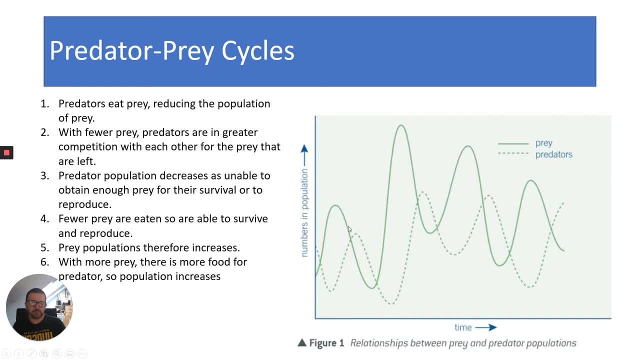 predators eat prey, they reduce. it reduces the population of the prey and the population of the predator increases predators population will decrease eventually as there's not enough prey to allow that population of predators to remain, so few prey are eventually eaten and therefore they survive and reproduce and therefore increase the prey population. so with 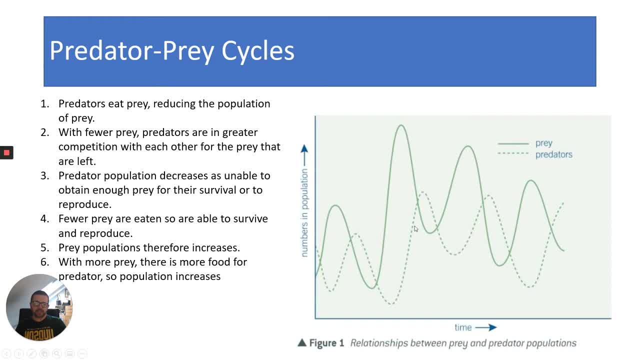 more prey, there is more food for predators, so populations then increase. you can see there's a lag between prey and predator, so predator always lags behind the prey in an exam. they might ask you to describe graphs. they might ask you to talk about this particular lag between prey and predator. now this: 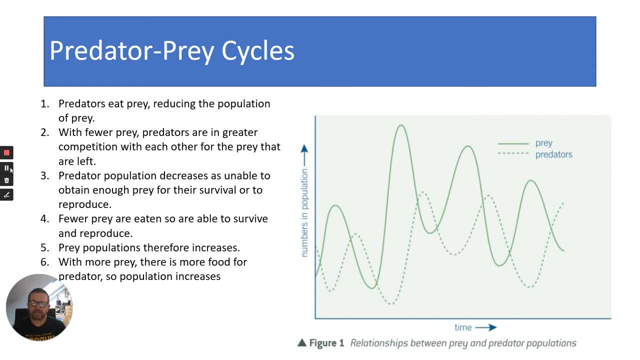 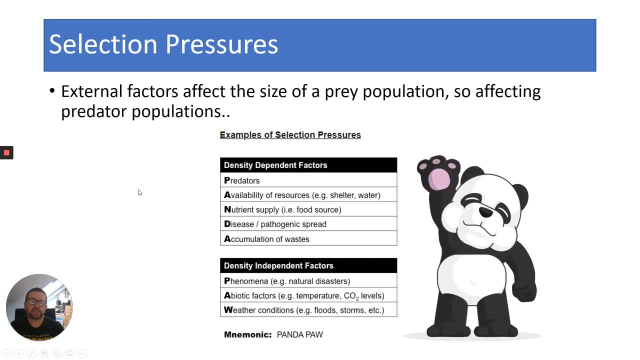 isn't straightforward. I mean, obviously there are other factors externally that are going to affect prey and predator species populations and those are called selection pressures. so external factors affect the size of a prey population, so affecting the predator population. so in your spec in AQA you don't need to know about density. 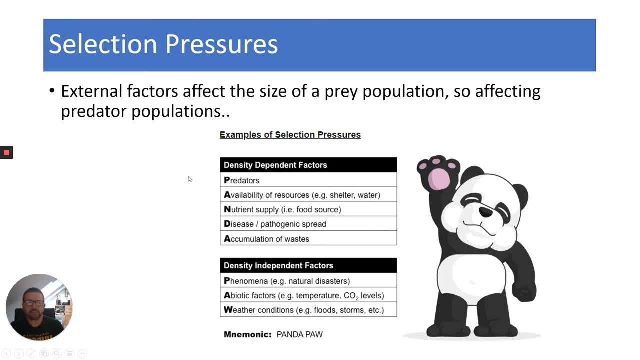 dependent and density independent factors. but it's worth knowing what other factors would affect predator prey relationships and particularly, for example, nutrient supply, but also things like disease and pathogenic spread accumulation and the waste. if the populations are too large, and then other things like natural disasters- you might get extremes of weather conditions and also abiotic. 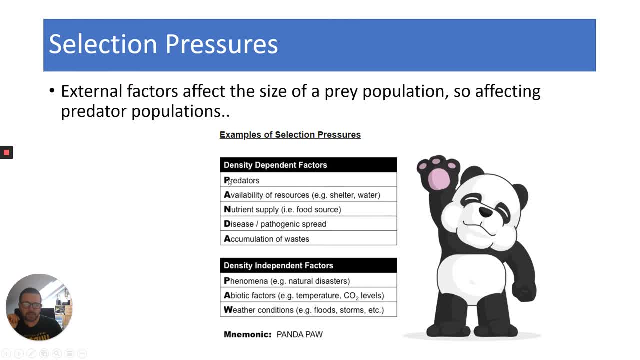 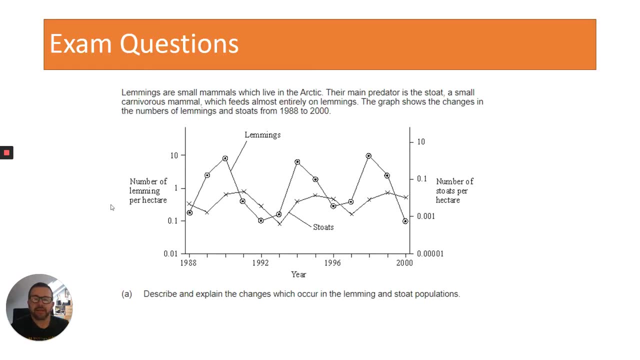 factors affecting. you can remember the selection pressures through this mnemonic. and it's panda paw, very interesting, okay, so let's have a look at some exam questions. so I'm going to show you an exam question. so, for example, this exam question: okay, and what I would like you to do. 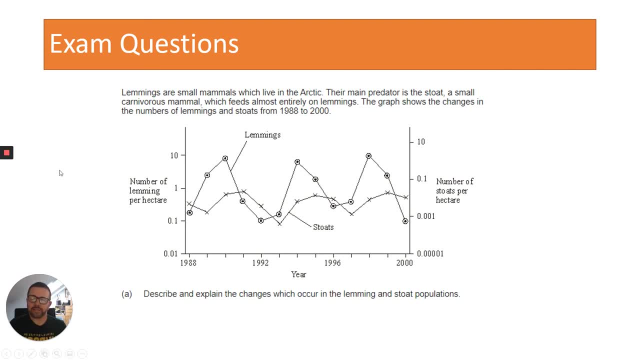 is to have a read and pause and see if you can answer it. before you do that, though, let's talk about what it wants you to show, so this is a six Mark question here, so they show you some information about some lemmings and stoats, and they 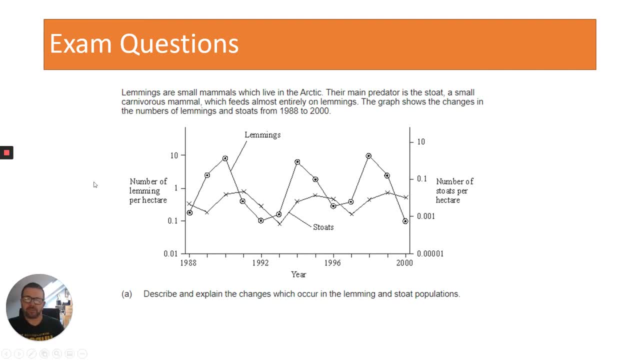 talk about the changes in the number of lemmings and stoats from 1988 to 2000, so a nice scale. on the bottom of years they show the number of stoats and the number of lemmings, uh, and it's mapped out and they say: describe and explain the changes which occur in the. 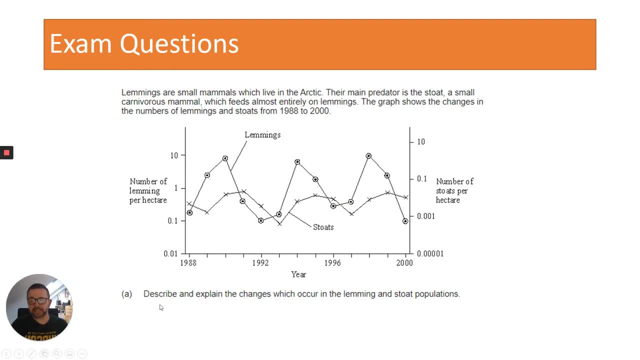 lemming and stoke population. so just a reminder: describe is is actually describing the curve. okay, now, obviously there's a lot going on between the lemmings and stoats. you need to describe it as simply as you can and then explain means give a biological reason why so I'd like you to pause. 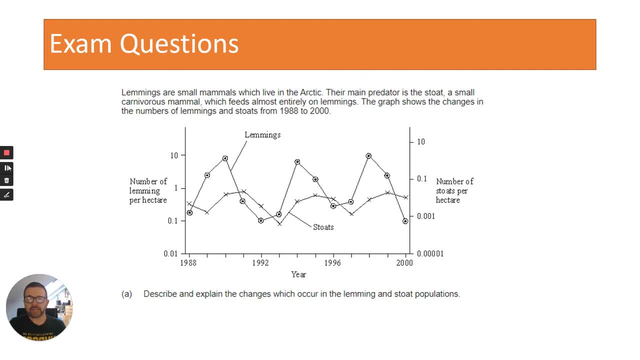 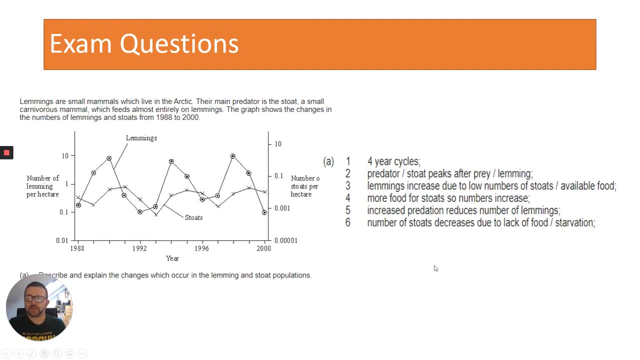 and see how you get on with the answer once you've finished press play. okay, so let's have a look at the answers. so the first thing to say about describing- I'll move myself over there, uh, describing. so if you look, there's uh, you can see there is a four year cycle, so meaning that the cycle 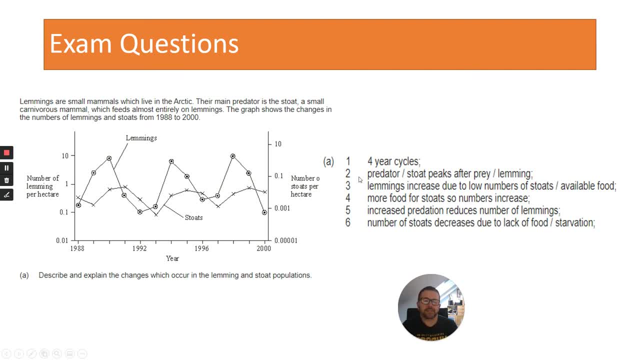 changes every four years. so predators, uh. the stoat peaks after the prey, so that's that lag. so the numbers peak after the prey. Lemmings increase due to low numbers of stoats, so they increase because numbers are decreasing, so lemmings increase. There's more food for stoats, so the 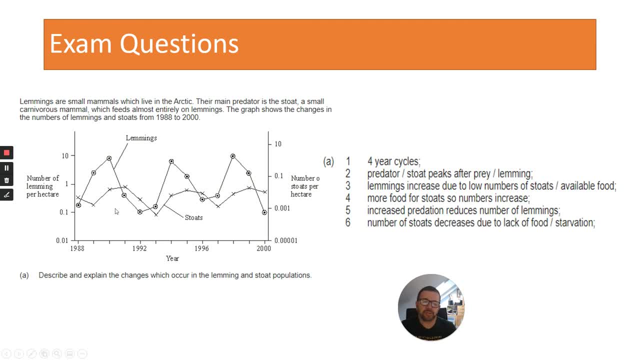 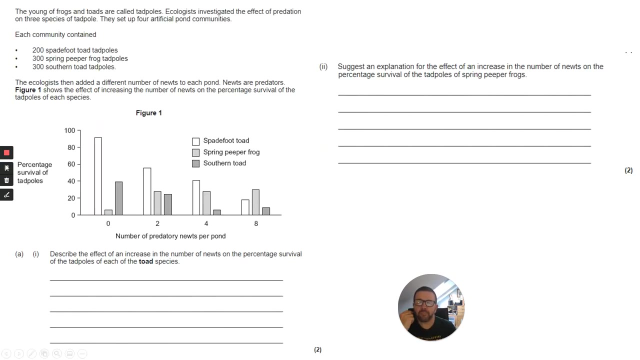 numbers will then increase. An increased predation reduces the number of lemmings and the number of stoats decreases due to the lack of food or starvation. So it's a simple description and explanation. Okay, so some questions are not just about describing but suggesting explanations. 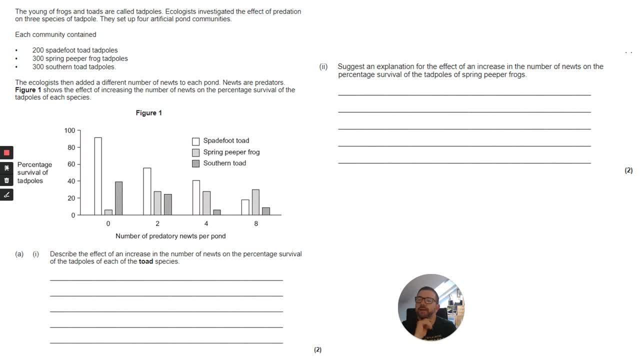 as well. So this is quite an interesting question about young frogs and toads and investigating the effect of predation on three species of tadpoles. So they set up four artificial pond communities and each community tells you each community. and then they added: 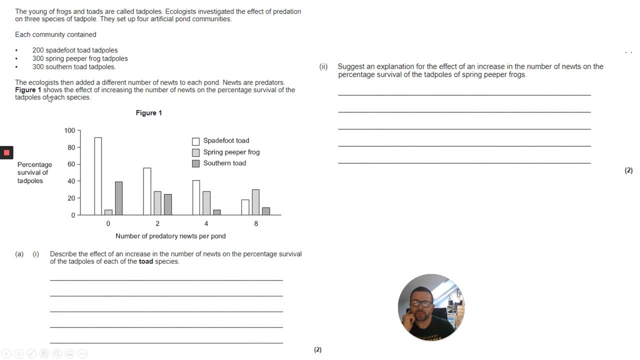 a different number of newts to each pond. okay. and then newts are predators and it shows the effects of increase in the number of newts on the percentage survival of the tadpole of each species. so it actually shows the number of predatory newts per pond on the x-axis and 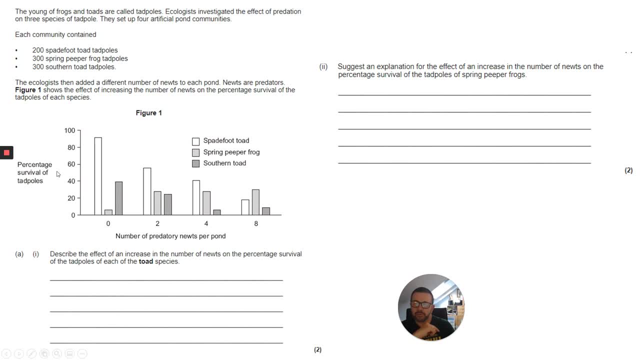 the percentage survival of tadpoles on the y. so first question it says: describe the effect of an increase in the number of newts on the percentage survival of the tadpoles of each of the toad species. notice toad is in bold. that means you are just looking at the spadefoot toad. 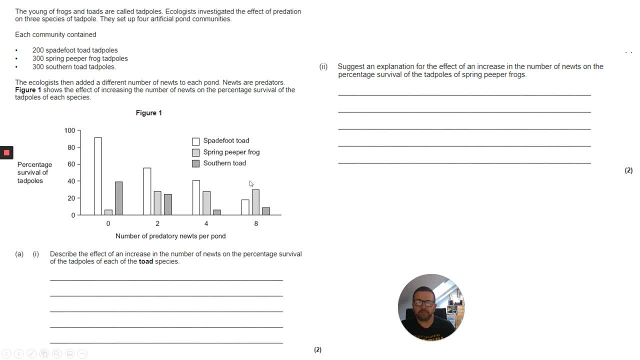 and the southern toad. you're not looking at the spring peeper frog, so it's really important to pick up on that. that they just want you to talk about the toad species. so, again, pause and see how you get on. i'd like you to try and answer that and then we will go through the answer. 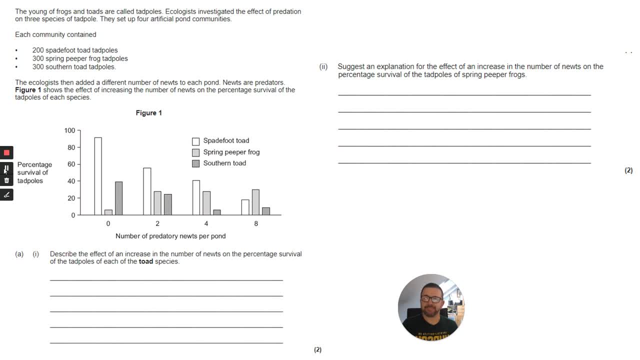 so pause now. okay, so remember a description. so description of each toad species, so spadefoot toad species, is quite easy, because as the number of newts increases, the number of spadefoot toads decreases. we then look at the spring- uh sorry, the southern toad- and you see, the southern toad decreases down. 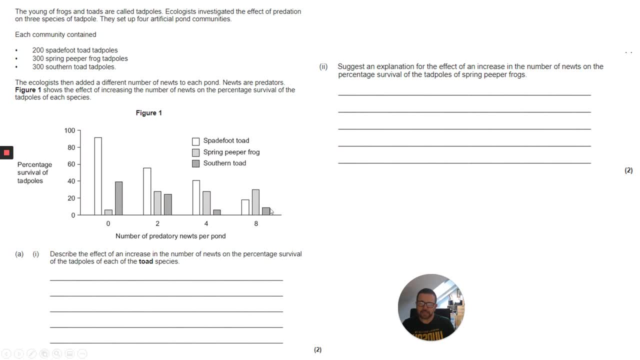 to where there is four predatory newts and then it slightly increases. so decreases in spade foot toad and decrease in southern toad up to four newts per pond. then it increases at eight newts per pond. so that's just a description of what you can see. 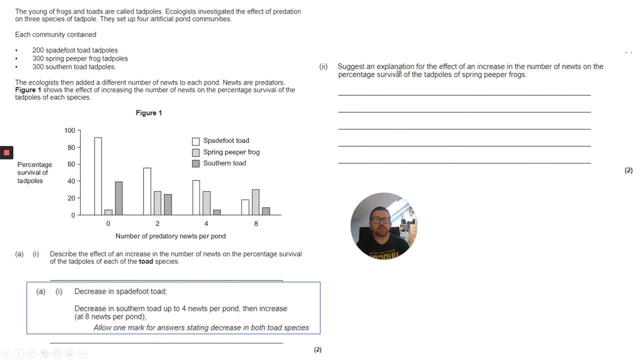 so the question then goes on to ask you suggest an explanation for the effect of an increase in the number of newts on the percentage survival of the tadpoles of spring peeper frogs. so again, i'd like you to pause the video and have a go at the answers. so pause and see how the description goes. 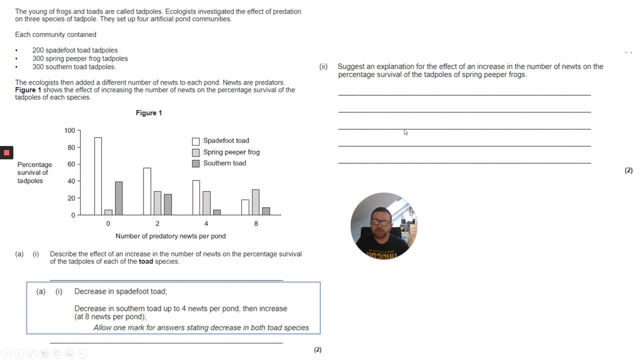 Now, OK. so looking at the graph for spring peeper frogs, you can see that actually the numbers are quite. they actually increase and they stay quite stable, even though the number of predatory newts increases. So what it would suggest is that the predatory newts are not eating the spring peeper frog tadpoles. 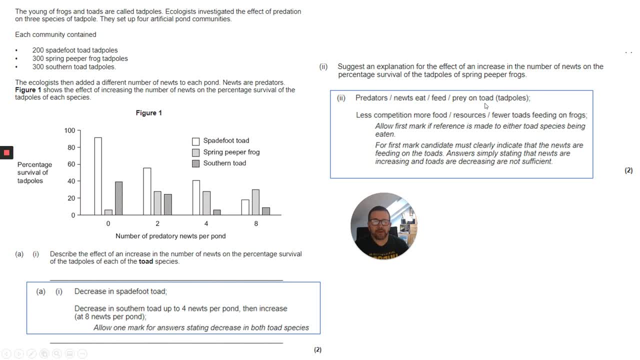 So the predators are not eating, they're preying on the toads. Therefore there is less competition for the spring peeper frog tadpoles, So there's fewer toads also feeding on frogs as well, because toads feed on frogs. but there's less competition and there's more food. 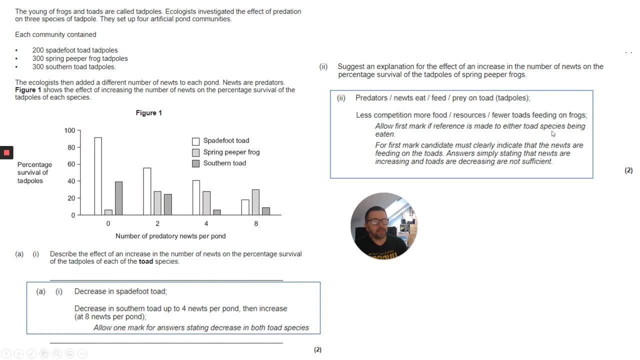 OK. so it says here: allow first mark if reference is made to either toad species being eaten by the newts. The answer simply states that newts are increasing and toads are decreasing and not sufficient. So you've got to give a bit more detail. 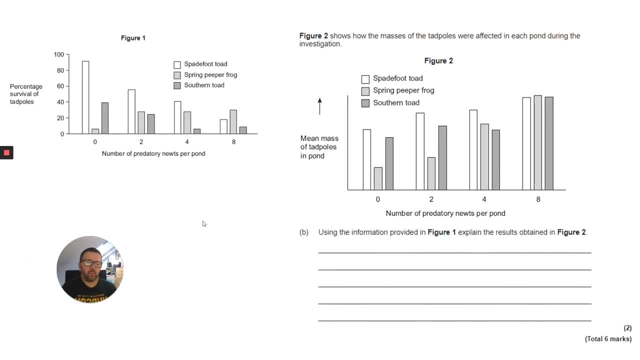 OK, so this next question is using both figure one and figure two. and figure two shows how the masses of the tadpoles were affected in each pond during the investigation. So you can see the mean mass tadpole on the y-axis. So, spadefoot toad, you can see the mass slightly increased.